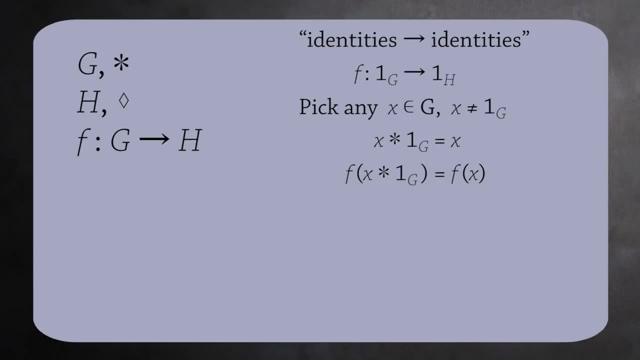 Since f is a homomorphism, we can write the left side as f of x times f of 1 sub g. Now f of x is an element in h. Let's call it y. This gives us y times f of 1 sub g equals y. 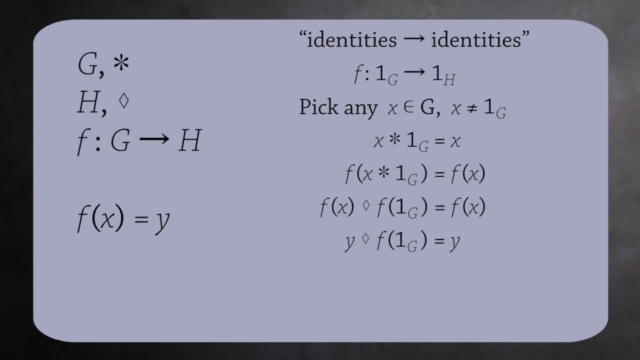 And since h is a group, y has an inverse. If we multiply both sides by the inverse of y, we get f of 1 sub g equals 1 sub h. This proves that homomorphisms send identity elements to identity elements. 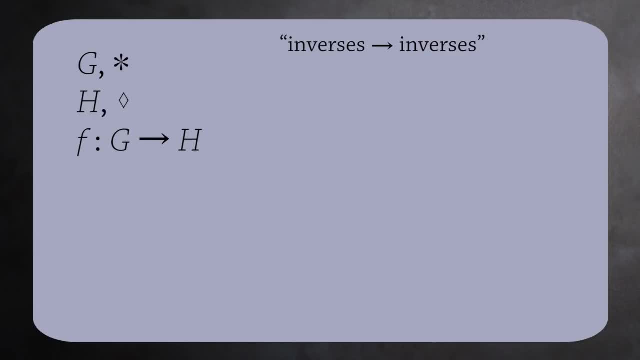 Next, we'll show why homomorphisms send inverses to inverses. Suppose f of x equals y. Note that x is in g and y is in h. We want to show that f of x inverse equals y inverse. To see why, we'll use the fact that x times x inverse equals 1 sub g. If you apply f to both sides, you get f of x times x inverse equals f of 1 sub g. We just showed that f of 1 sub g equals 1 sub h. And on the left, we can use a property of homomorphisms to get f of x times f of x inverse equals 1 sub h. f of x equals y, so we get y times f of x inverse equals 1 sub h. Multiplying both sides on the left by y inverse gives us f of x inverse equals y inverse. 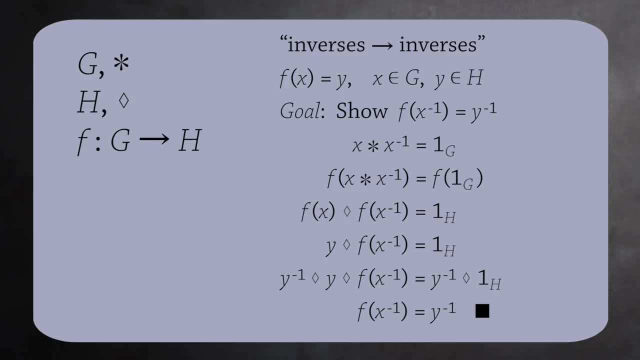 This proves that homomorphisms send inverses to inverses. 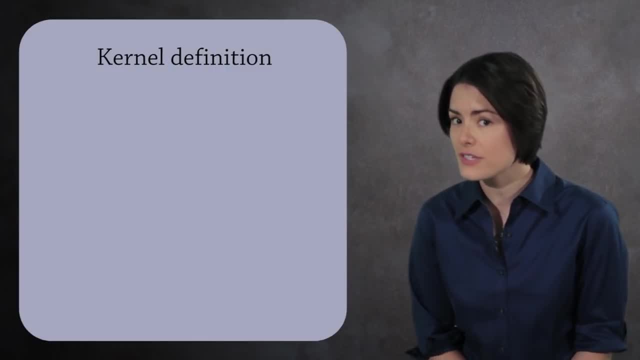 We now have all the tools we need to define homomorphisms. First, we need to understand the kernel. Suppose that f is not 1 to 1. 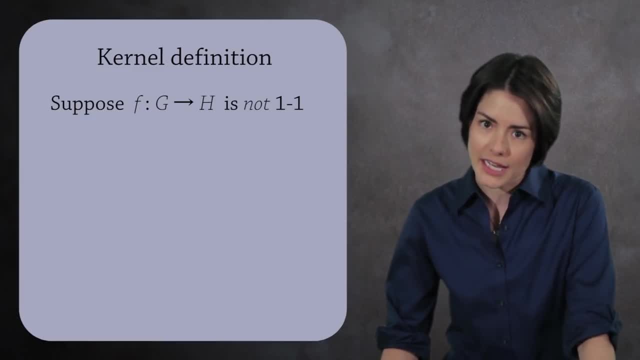 Then there are at least two elements in g which map to the same element in h. 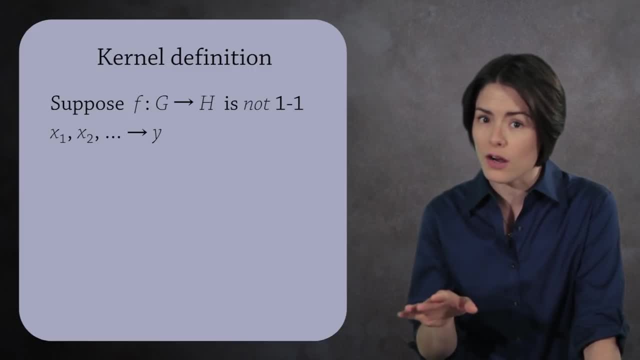 To be concrete, suppose x1, x2, and so on are the elements which map to y. This means f of x1 equals y, f of x2 equals y, and so forth. 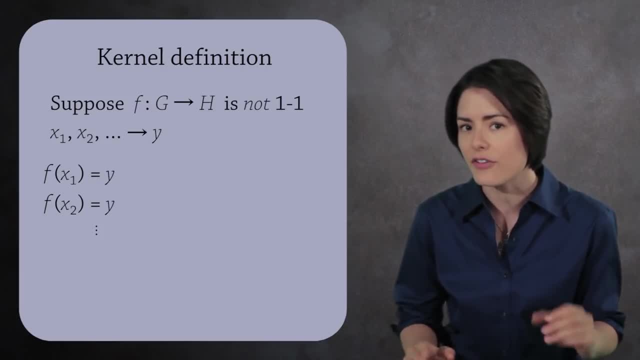 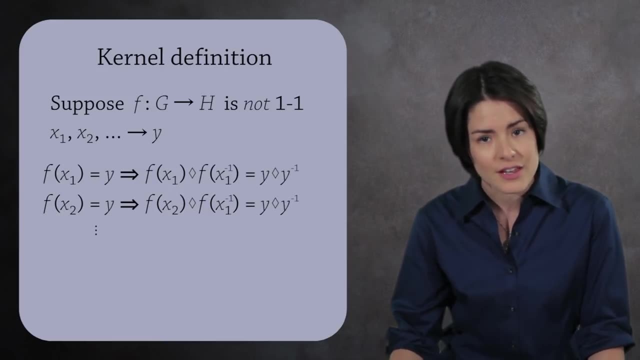 Now watch what happens if we multiply all of these equalities by f of x1 inverse. Since homomorphisms send inverses to inverses, f of x1 inverse equals y inverse. This allows us to identify the right-hand sides. Next, we can combine the left-hand sides because f is a homomorphism.